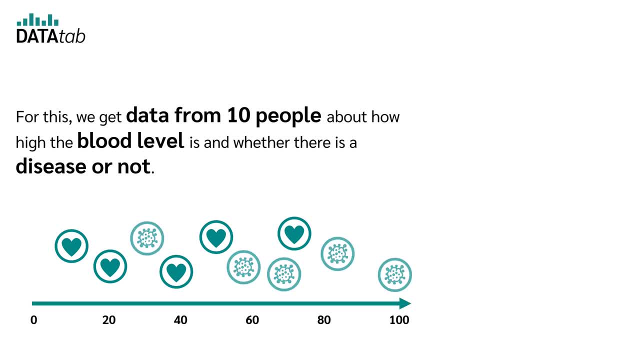 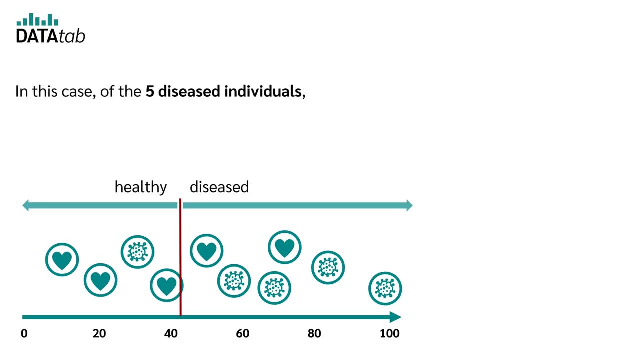 how high the blood level is and whether there is a disease or not. We could now choose a classification threshold for a certain blood value. For this we get data from 10 people, that this person has cancer or not. We would quickly need to select a prediction threshold. 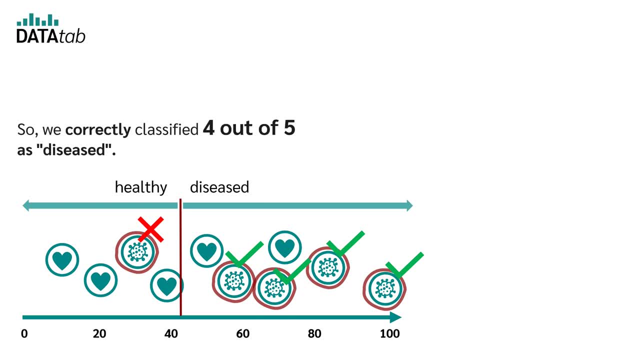 of 45.. For example, in this case, of the five diseased individuals, we would correctly classify four as diseased and one incorrectly as healthy. So we correctly classified four out of five as diseased. This value is called the true positive rate, TPR, and is equal to the sensitivity. 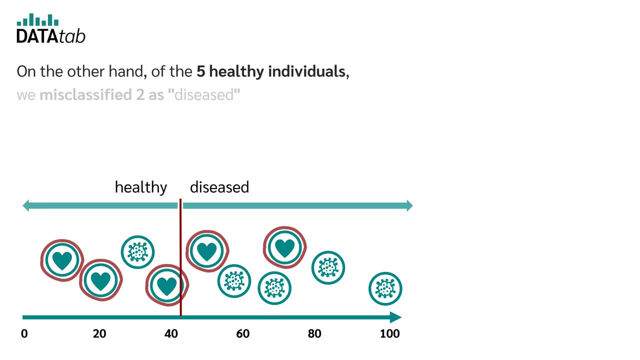 On the other hand, of the five healthy individuals, we make our conclusion that this person is misclassified 2 as diseased and correctly classified 3 as healthy. So we misclassified 2 out of 5 as diseased. This value is called the false positive rate, FPR, and is 1 minus. 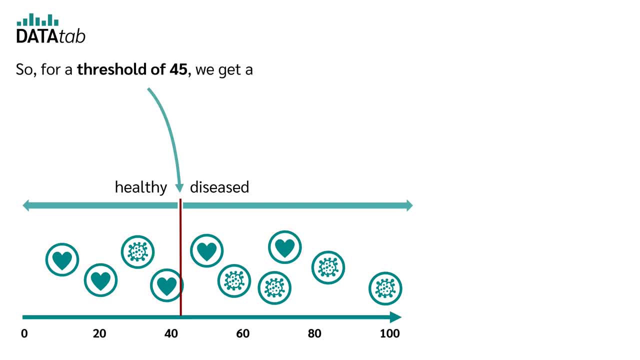 the specificity. So for a threshold of 45, we get a true positive rate of 4 out of 5, ie 0.8, and a false positive rate of 3 out of 5, ie 0.6.. The true positive rate is calculated with: 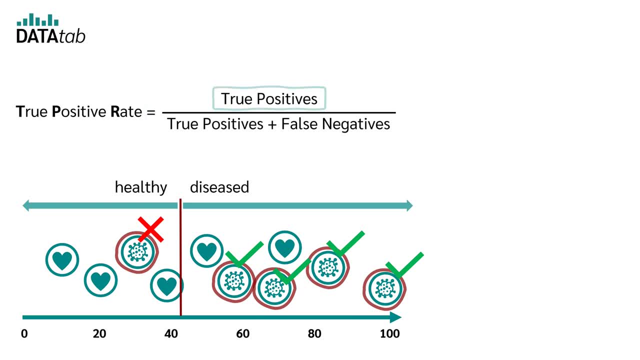 this equation, The true positive rate is equal to the true positives divided by the true positives plus the false negatives. The true positives are the people correctly classified as diseased and the false negatives are the people incorrectly classified as healthy. The false positive rate is obtained with this equation: The false positive rate is equal to the false positives. 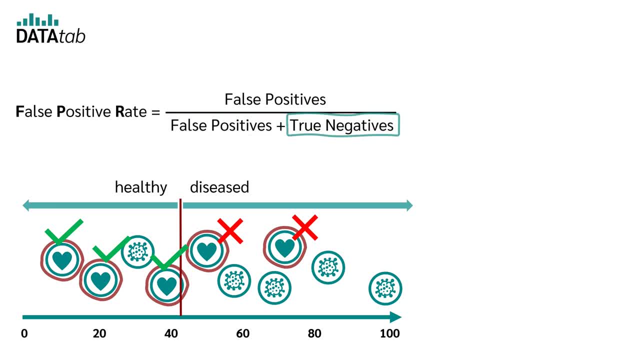 divided by the false positives plus the true negatives. The false positives are the healthy individuals misclassified as diseased, and the true negatives are the individuals correctly classified as healthy. We can now calculate, for each threshold, the true positive rate and the false positive rate, And it is precisely these two values that we are going to calculate. The values that are then plotted on the ROC curve. The true positive rate is plotted on the y-axis and the false positive rate on the x-axis. Now let's draw the complete ROC curve. for our example, If we choose the threshold value to be very small, ie pushed all the way to the left. 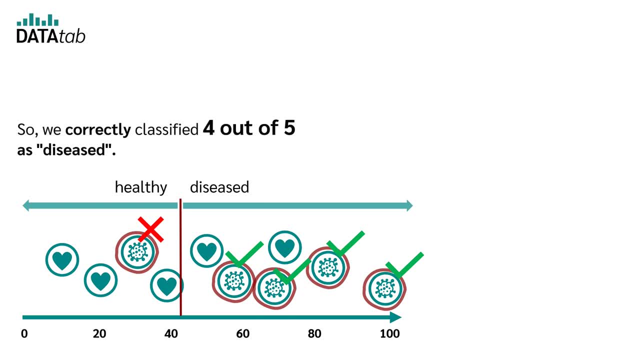 and 1 incorrectly as healthy, So we correctly classified 4 out of 5 as diseased. This value is called the true positive rate, TPR, and is equal to the sensitivity. On the other hand, of the 5 healthy individuals, we misclassified 2 as diseased and correctly. 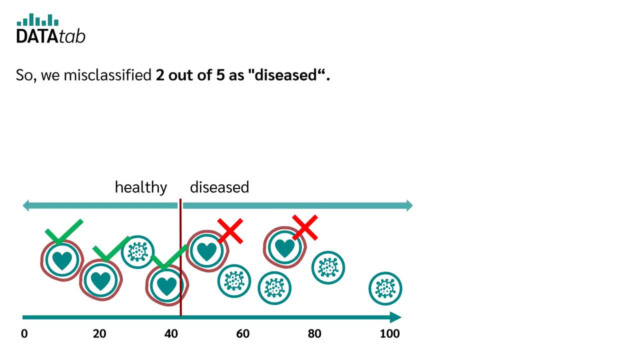 classified 3 as healthy, So we misclassified 2 out of 5 as diseased. This value is called the false positive rate, FPR, and is 1 minus the specificity. So for a threshold of 45, we get a true positive rate of 4 out of 5,, ie 0.8 and a false positive. 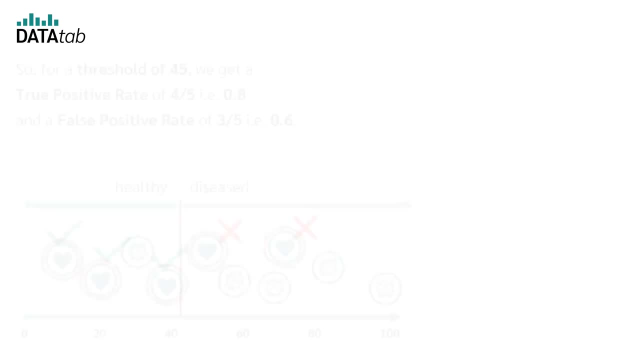 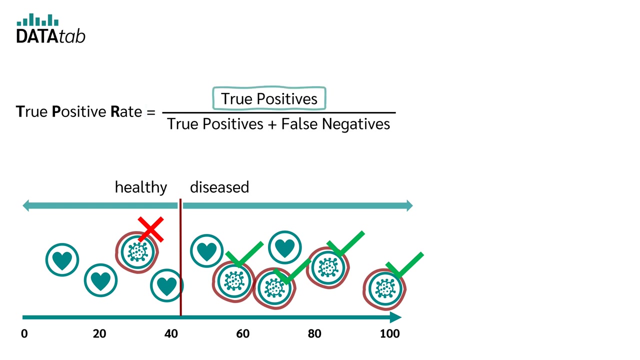 rate of 3 out of 5,, ie 0.6.. The true positive rate is calculated with this equation: The true positive rate is equal to the true positives divided by the true positives plus the false negatives. The true positives are the people correctly classified as diseased and the false negatives 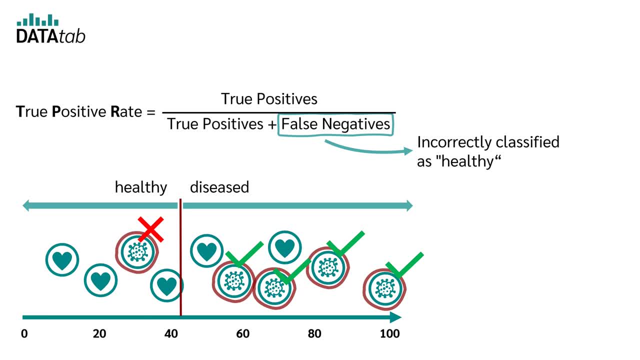 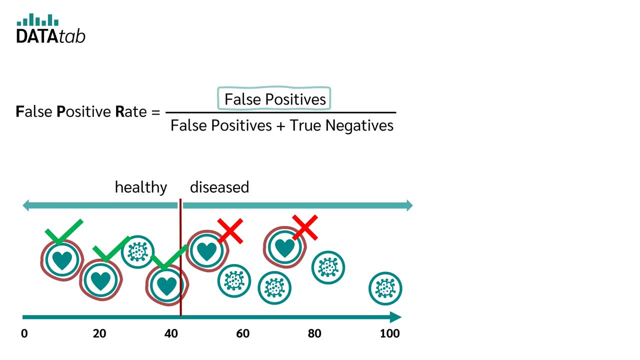 are the people incorrectly classified as healthy. The false positive rate is obtained with this equation: The false positive rate is equal to the false positives divided by the false positives plus the true negatives. The false positives are the healthy individuals misclassified as deceased and the true negatives are the individuals correctly classified as healthy. 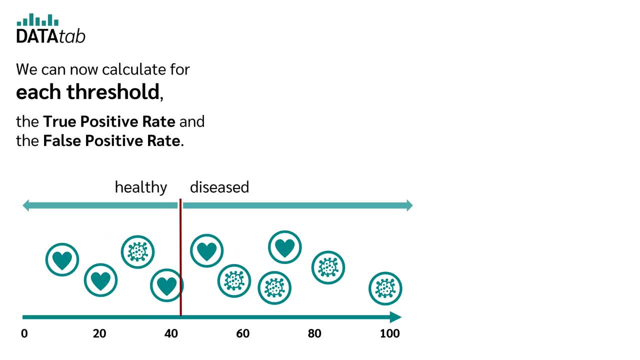 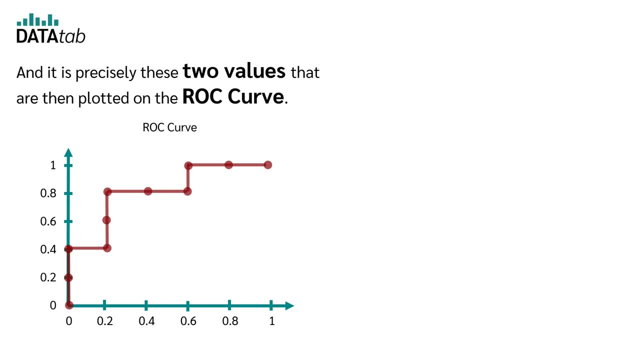 We can now calculate, for each threshold the true positive rate and the false positive rate, And it is precisely these two values that are then plotted on the ROC curve. The true positive rate is plotted on the y-axis and the false positive rate on the x-axis. 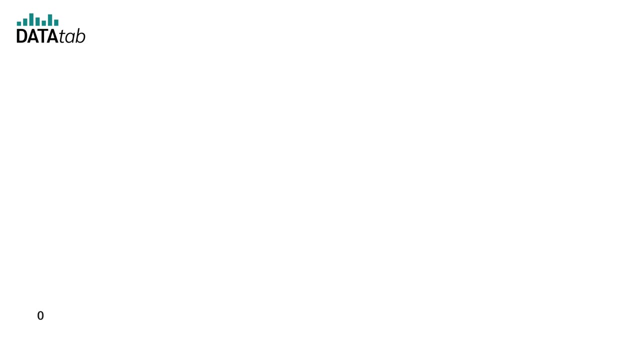 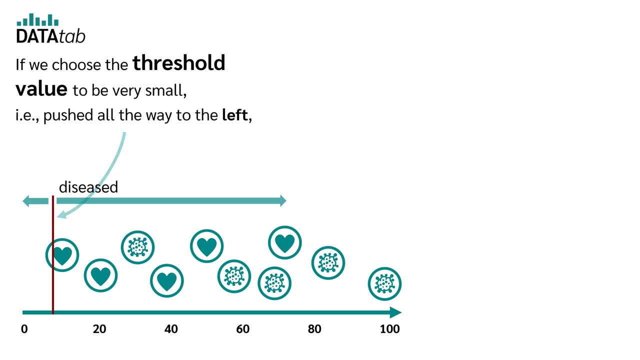 Now let's draw the complete ROC curve. for our example. If we choose the threshold value to be very small, ie pushed all the way to the left, we correctly classify all five deceased individuals. Our true positive rate is thus 5 out of 5, ie 1.. 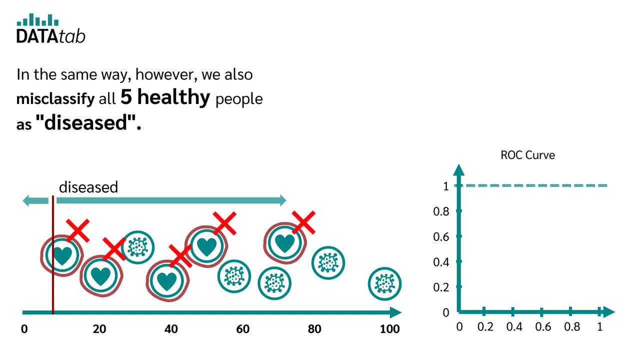 In the same way, however, we also misclassify all five healthy people as deceased. Our false positive rate is thus 5 out of 5, ie 1.. With that we have the first point. Now we can push the threshold further. 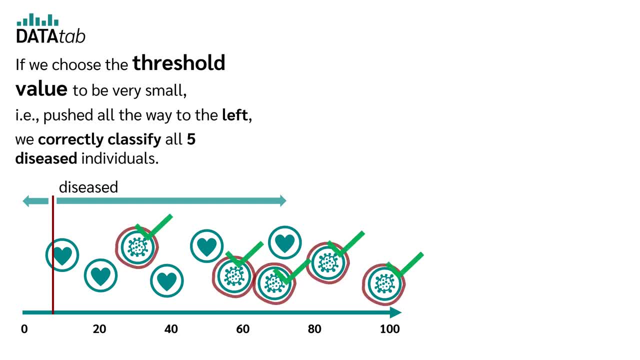 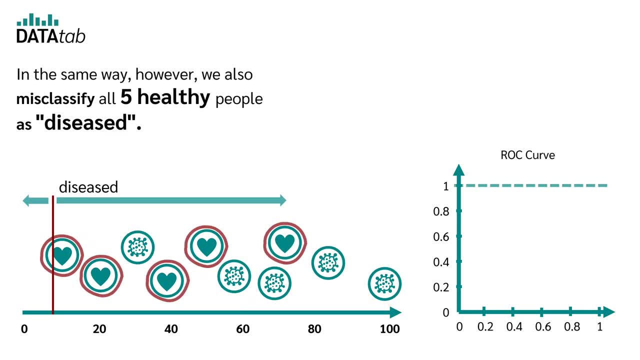 we correctly classify all five diseased individuals. Our true positive rate is thus 5 out of 5, ie 1.. In the same way, however, we also misclassify all five healthy people as diseased. Our false positive rate is thus 5 out of 5, ie 1.. With that we have the first point. 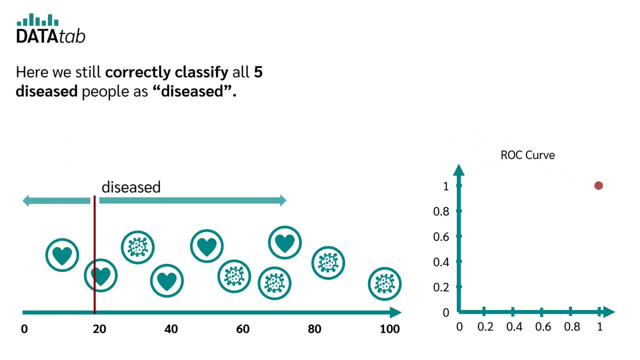 Now we can push the threshold further Here. we still correctly classify all five diseased people as diseased. So we continue to have a true positive rate, 5 out of 5.. However, of the 5 healthy individuals, we now misclassify only 4 out of 5 as diseased. 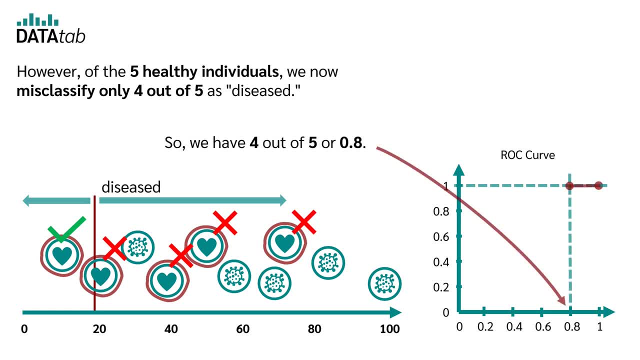 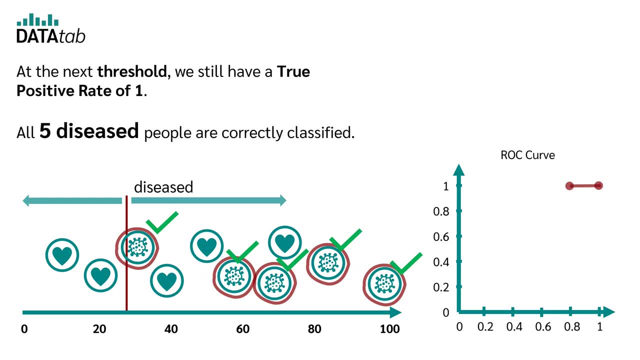 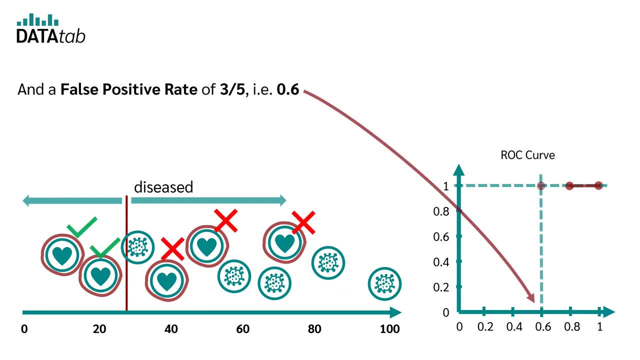 So we have 4 out of 5 or 0.8.. At the next threshold we still have a true positive rate of 1.. All 5 diseased people are correctly classified And a false positive rate of 3 out of 5, ie 0.6.. 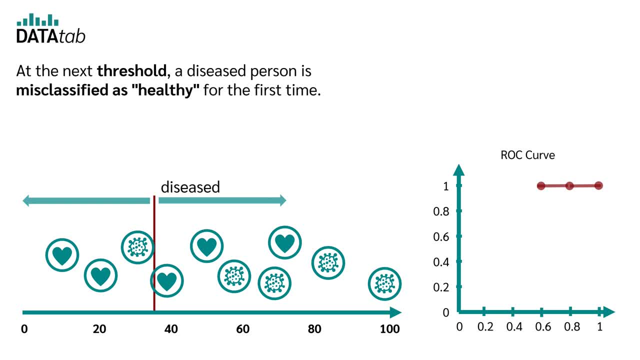 At the next threshold, a diseased person is misclassified as healthy for the first time. We therefore obtain a true positive rate of 4 out of 5, ie 0.8.. And a false positive rate of 3 out of 5, ie 0.6.. 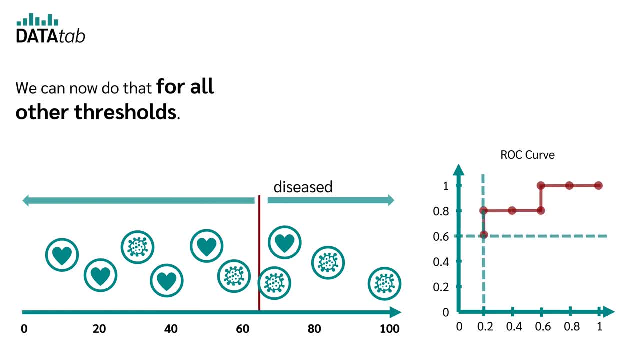 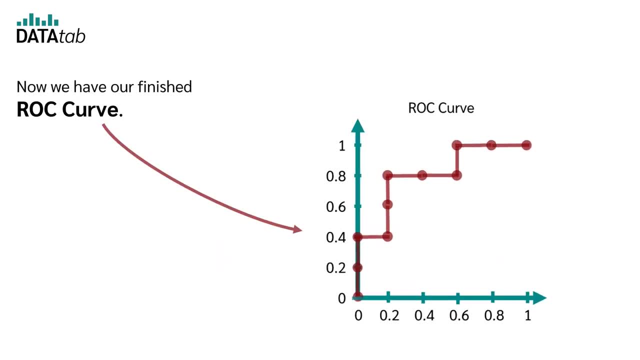 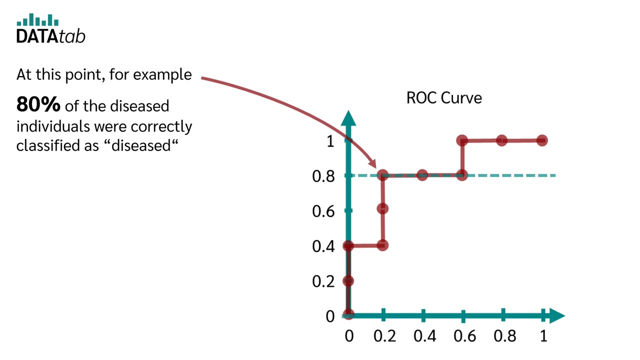 We can now do that for all other thresholds Now we have our finished R-O-T At this point. for example, 80% of the diseased individuals were correctly classified as diseased and 20% of the healthy individuals were incorrectly assigned diseased. 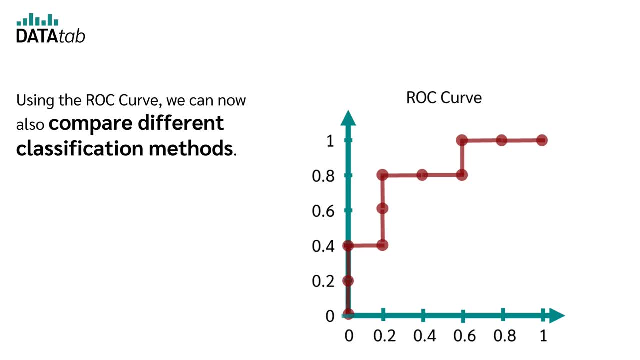 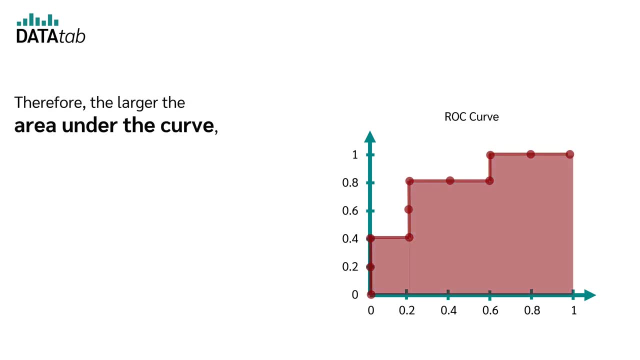 Using the R-O-T curve, we can now also compare different classification methods. A classification model is better the higher the curve is. Therefore, the larger the area under the curve, the better the classification, And it is precisely this area that is reflected by the A-U-C value: the area under the curve. 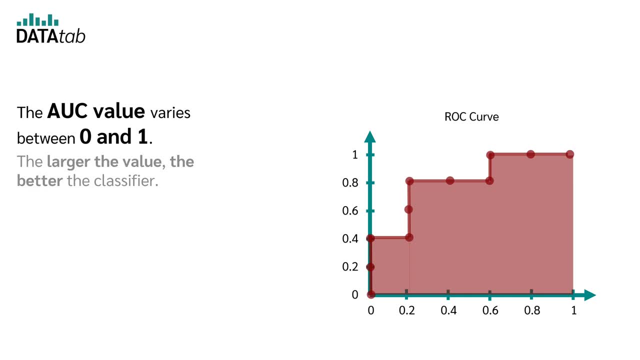 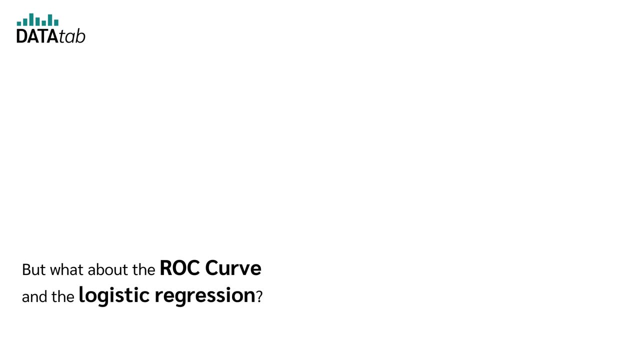 The A-U-C value varies between 0 and 1.. The larger the value, the better the classifier. But what about the R-O-C curve and the logistic regression? For example, we could build a new classification model using a logistic regression. 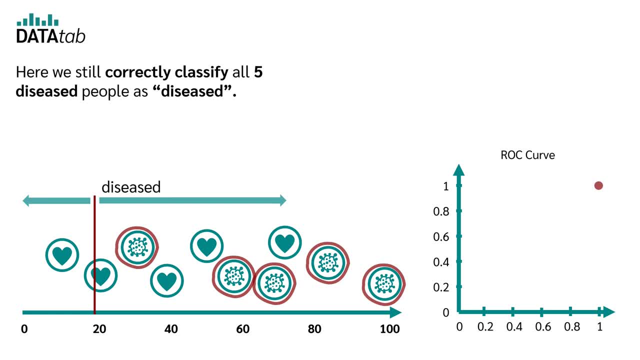 Here we still correctly classify all five deceased people as deceased, So we continue to have a true positive rate: 5 out of 5.. However, of the five healthy individuals, we now misclassify only 4 out of 5 as deceased. So we have 4 out of 5, or 0.8.. 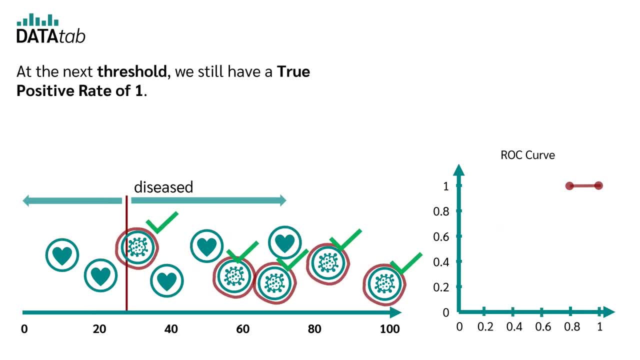 At the next threshold, we still have a true positive rate of 1.. All five deceased people are correctly classified And a false positive rate of 3 out of 5,, ie 0.6.. At the next threshold, a deceased person is misclassified as healthy for the first time. 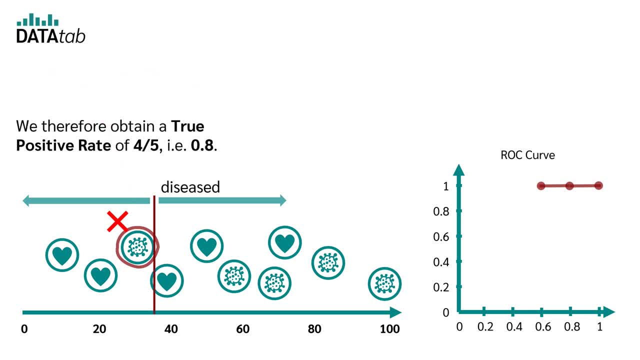 We therefore obtain a true positive rate of 4 out of 5, ie 0.8.. And a false positive rate of 3 out of 5, ie 0.6.. We can now do that for all other thresholds. 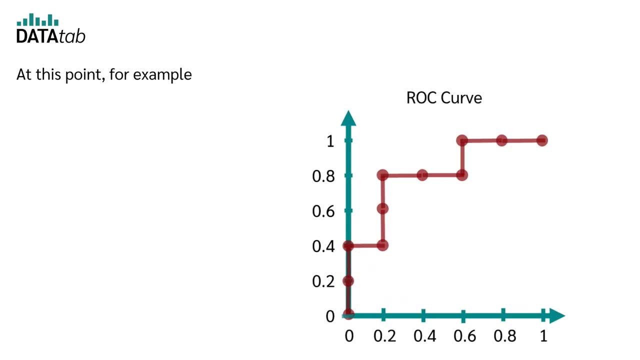 Now we have our finished ROC curve. At this point, for example, 80% of the deceased individuals were correctly classified as deceased And 20% of the healthy individuals were incorrectly assigned deceased. Using the ROC curve, we can now also compare different classification methods. 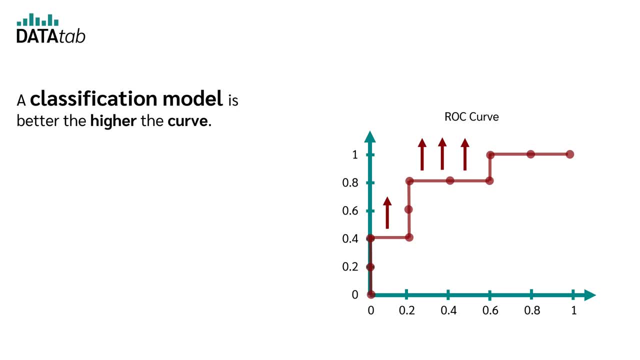 A classification model is better the higher the curve is. Therefore, the larger the area under the curve, the better the classifier is, And it is precisely this area that is reflected by the AUC: The area under the curve. The AUC value varies between 0 and 1.. 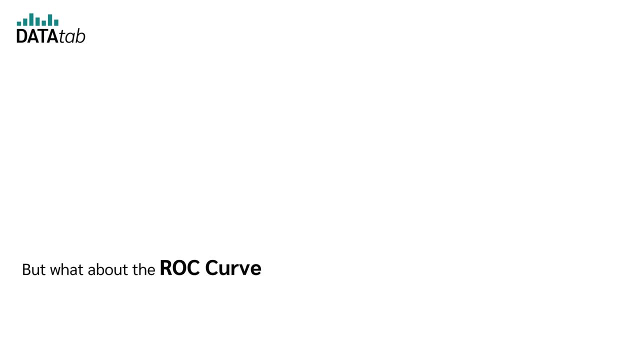 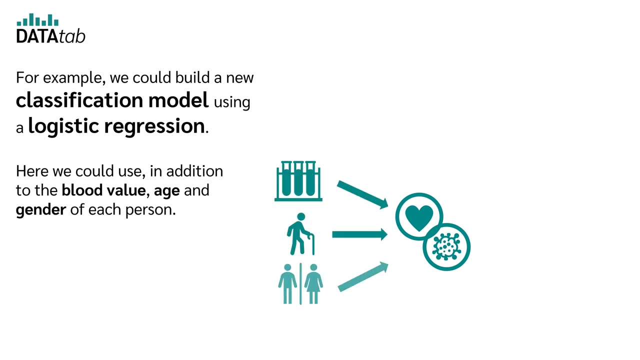 The larger the value, the better the classifier. But what about the ROC curve and the logistic regression, For example? we could build a new classification model using a logistic regression. Here we could use, in addition to the blood value, age and gender of a person. 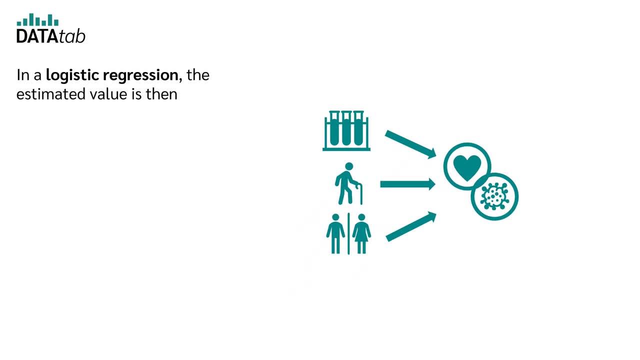 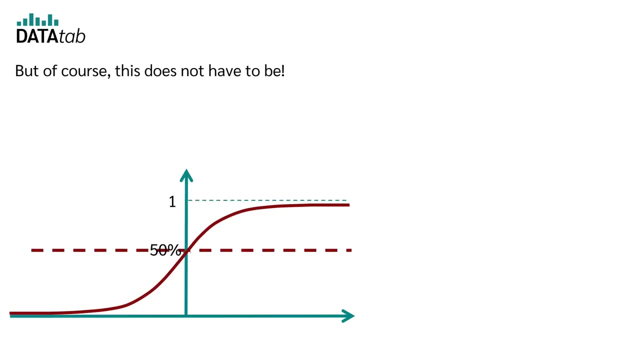 In a logistic regression. the estimated value is then how likely it is that a particular person is deceased. Very often, 50% is then simply taken as the threshold to classify whether a person is deceased or not, But of course this does not have to be.